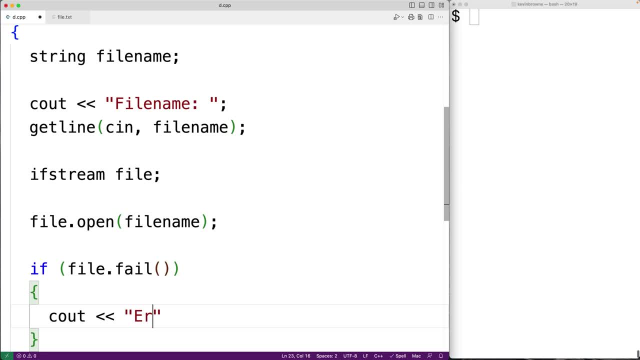 So we'll have here cout and then error opening file, followed by an end line, And we'll also have return one. Returning one instead of returning zero is a signal to the shell or the terminal that something has gone wrong in the execution of our program. 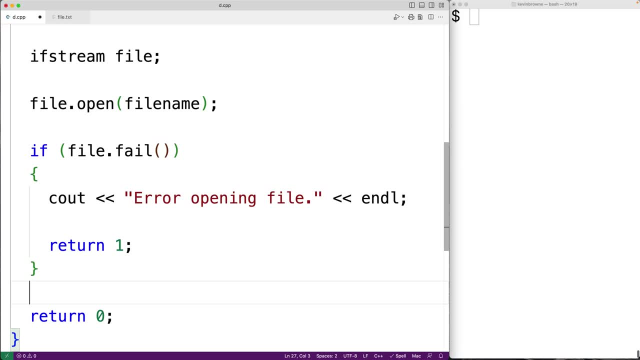 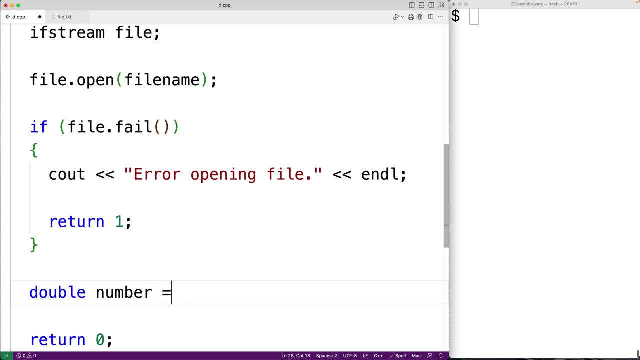 Now, at this point here we know the file has been opened correctly and we're ready to start reading in the numbers from the file. Let's create some variables to help with that. Here we'll have double number Where number is going to store each number that we read from the file. 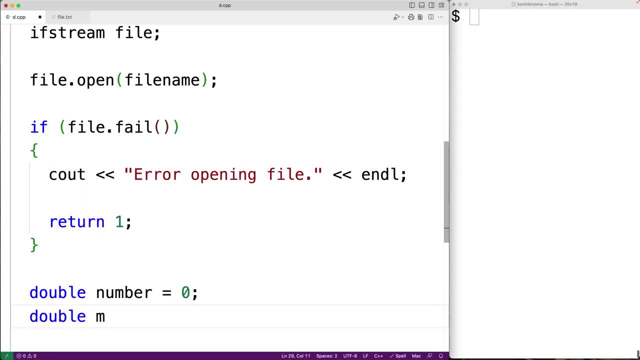 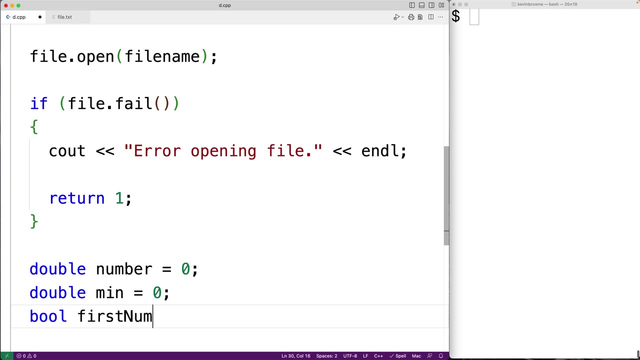 We'll then create a variable called min, And min is going to store the smallest number that we've found so far in the file. We'll create one more bool variable called first number, Because the first number that we read from the file is, by default, also going to be the. 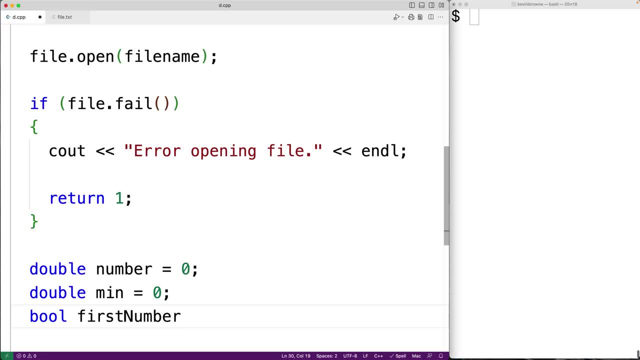 smallest number that we've found so far in the file. We'll assign the value true, And true is going to be used to indicate that we have not yet read in that first number from the file. We can now read in each number from the file: 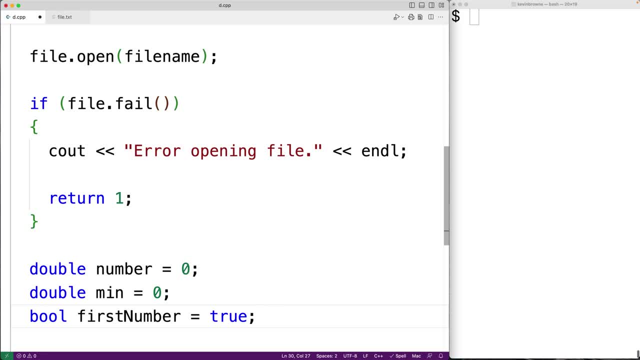 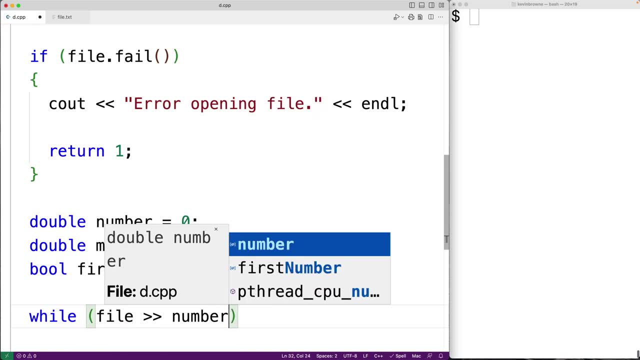 And we're going to update min accordingly. So we'll have here while file and then the stream extraction operator number. So this operation is going to read the next number in the file and store it into the number variable. The operation is going to evaluate to true. 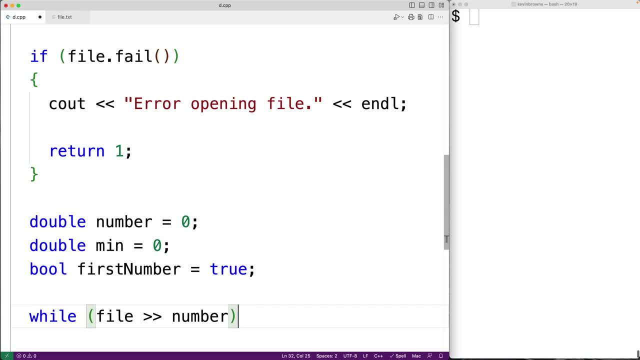 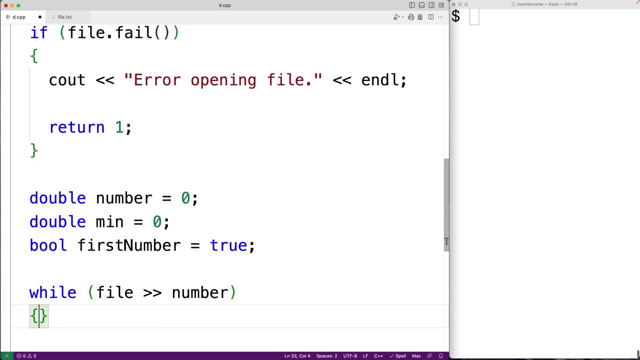 so long as a number has been successfully read from the file. So this loop is going to read in each number in the file until we reach the end of the file, at which point the operation is going to return false and the loop is going to stop. So in the loop body we'll have an if. 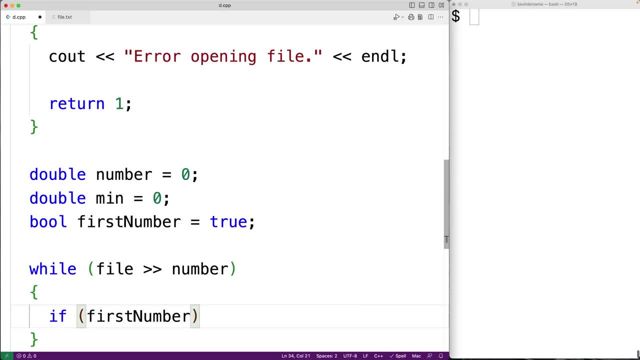 statement: if first number is true. So if first number is true, that means the number that we've just read in is the first number that we've actually read from the file, and if that's the case, by default, it is the smallest number that we've read from the file. So we'll have here. 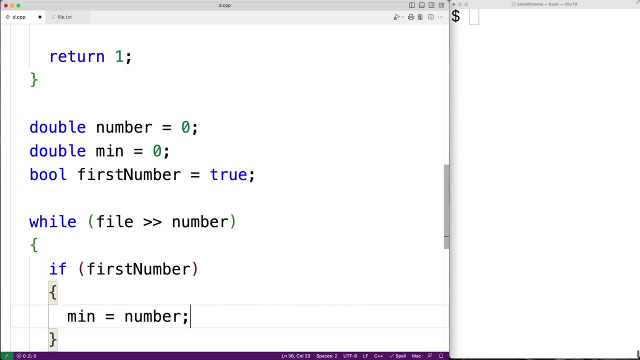 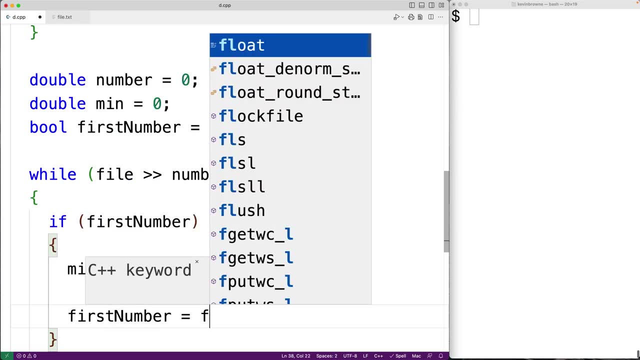 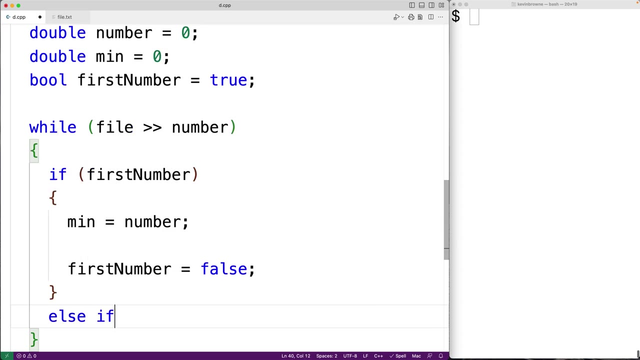 min is equal to number, We'll also assign false to first number to indicate that now we have read in the first number from the file. Otherwise, if first number is false, we'll check to see if the number is true. So, if first number is false, we'll check to see if the number is true. 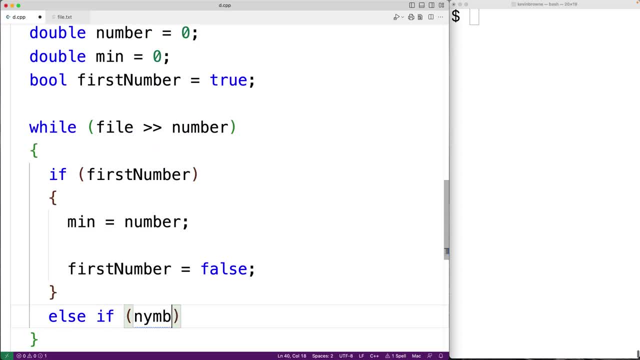 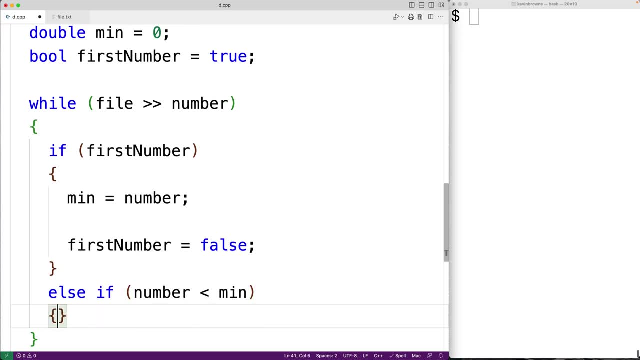 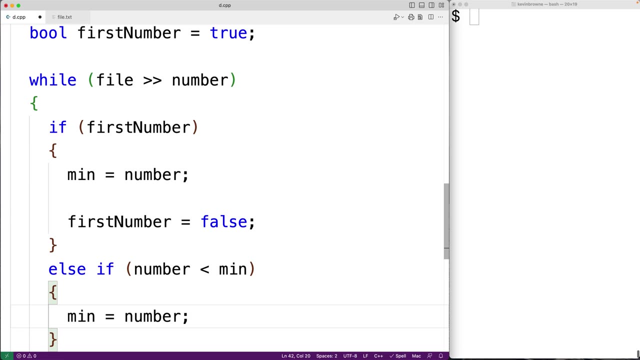 the number that we've just read in is less than min. If it is, we found a new smallest number and we need to update min. So we'll have here: min is equal to number to update min because here we found a new smallest number. So by the 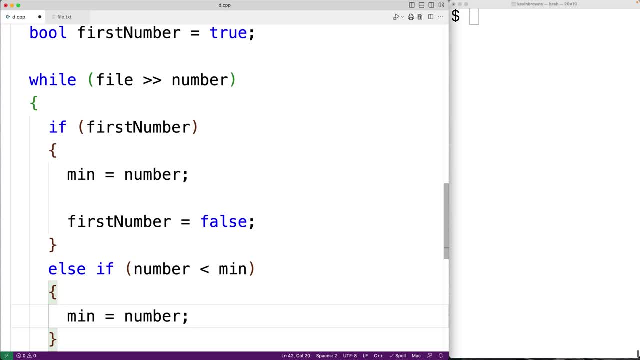 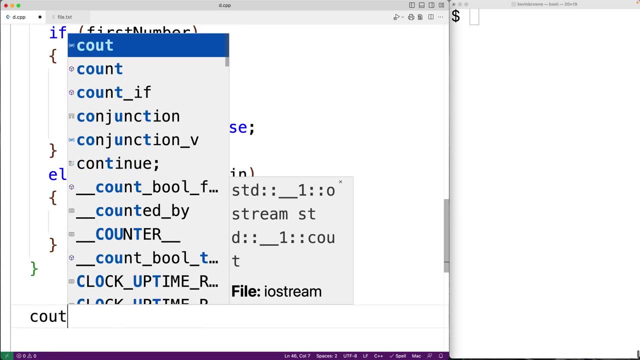 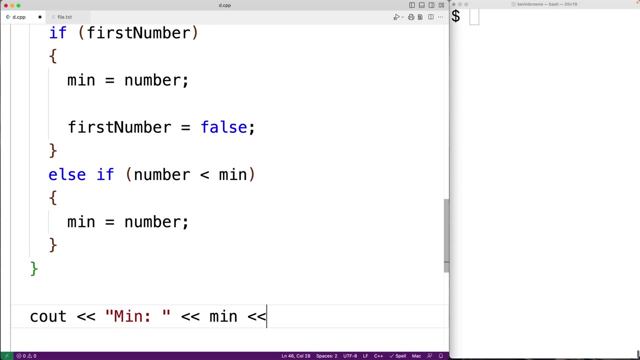 time this loop is done, min is going to be set to the smallest number that we found in the file. We can now output that number. So down here we could have cout and then min, colon and then min, followed by an end line. Now it is. 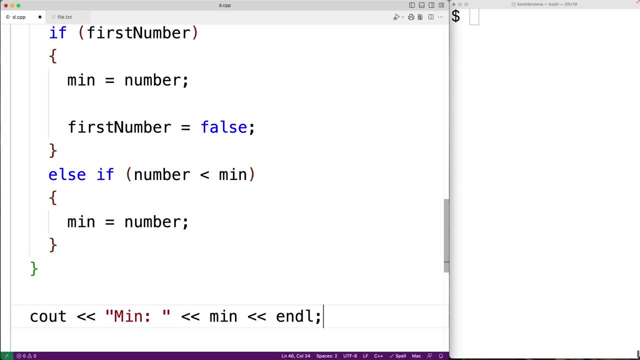 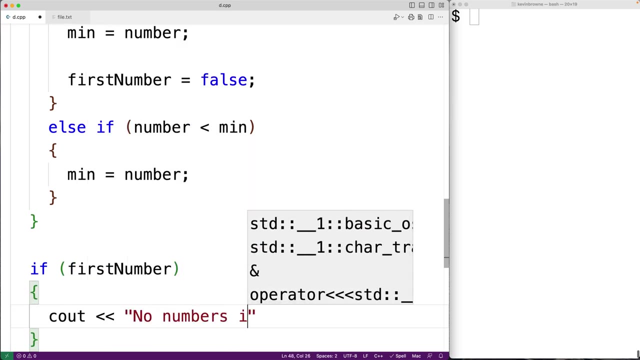 possible that the file contained no numbers at all. If that's the case, first number is still going to be set to true. We could handle that case We could have here. if first number is true, then we'll output no numbers in file, followed by an. 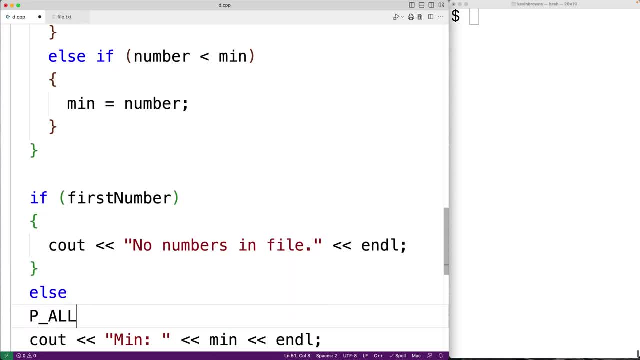 end line. Otherwise we'll output the min here and we'll just put the cout inside of here. Now the last thing we should do is close our access to the file. So here we'll have fileclose to close the file. We can now save our program and compile it. 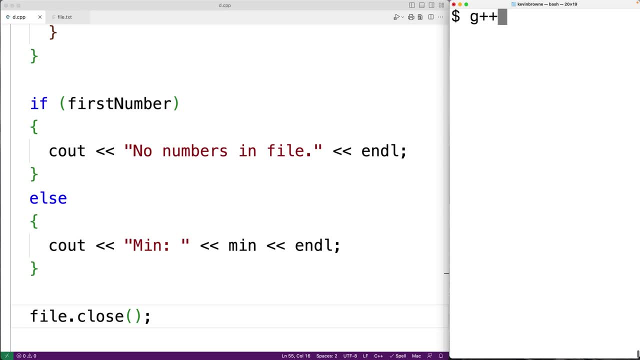 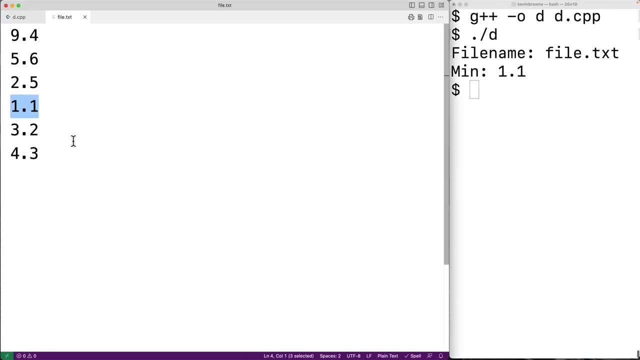 and test it out. So up here we'll first compile it and then we'll run it And I'll enter in filetxt for the file name and we get a min number of 1.1, which is correct, because 1.1 is the smallest number in that file. So this is how we can find the smallest. 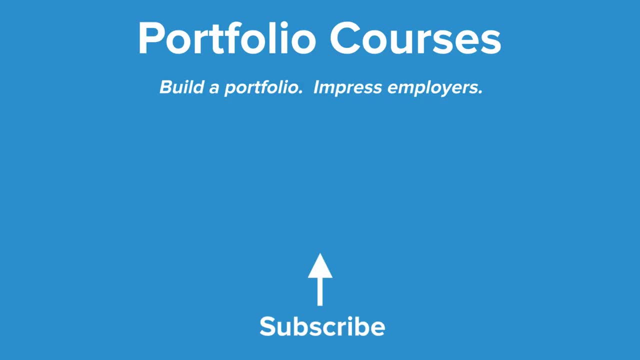 number in a file using C++. Check out PortfolioCoursescom, where we'll help you build a portfolio that will impress employers.